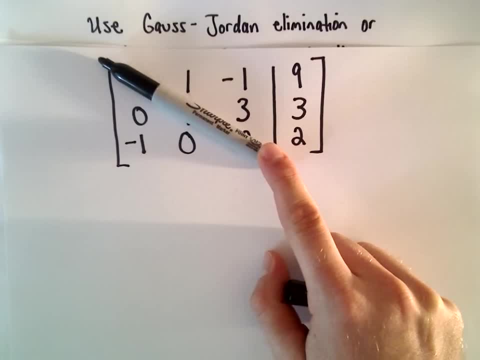 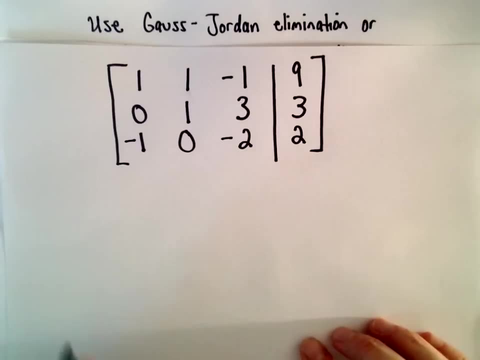 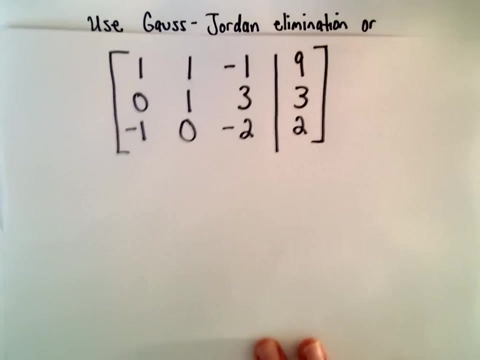 what we're shooting for here. okay, once we do that, we're gonna use some back substitution. so again, my goal eventually is to get zeros here, and I want ones along the diagonal. that's, that's our, that's what we're going for, okay, so that'll kind of be step one here. okay, so to get a zero in the in the third row. 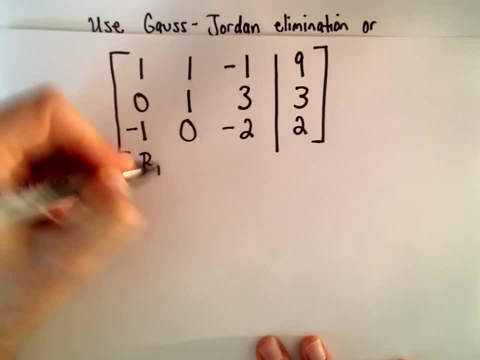 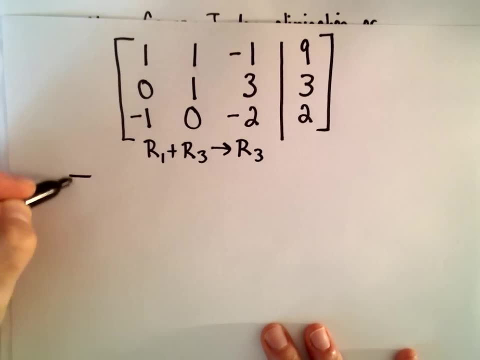 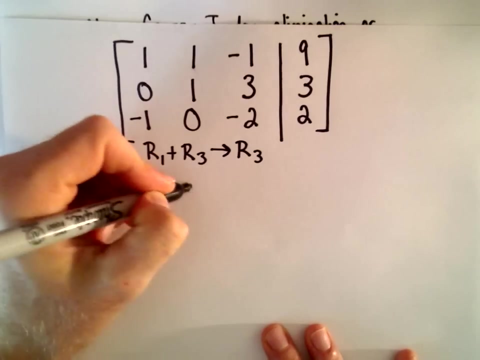 first column. I'm just gonna take row one and add that to row three and that's gonna replace my row three. I like to use the little arrow to indicate which row is changing. there's tons of arithmetic in these problems, so anything I can- you know I can do to help keep myself organized. I always found that helped. so 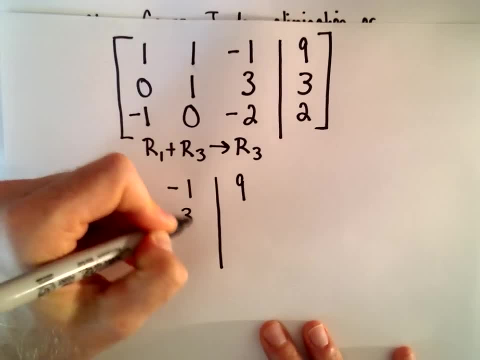 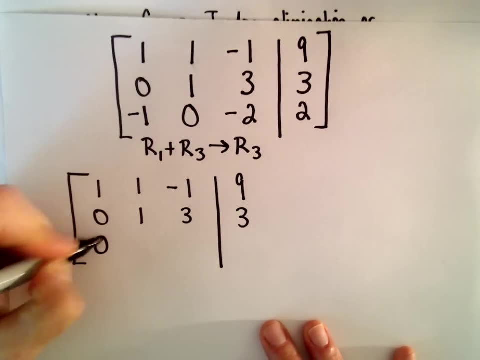 I'm not changing the first row, not changing the second row either, and that's what I'm going to do here. so I'm going to take my first row and I'm going to do my arithmetic, so one plus negative one will be zero. that's what we wanted. 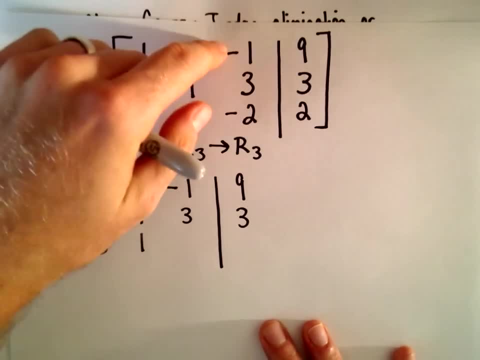 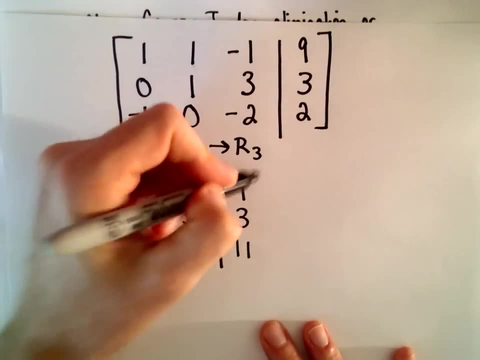 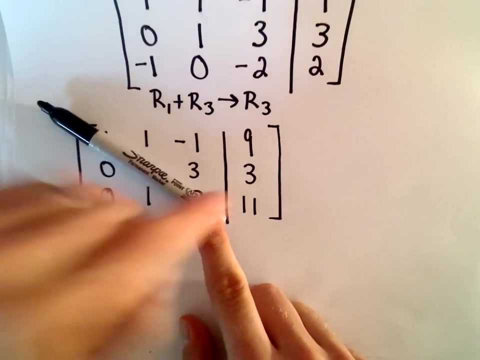 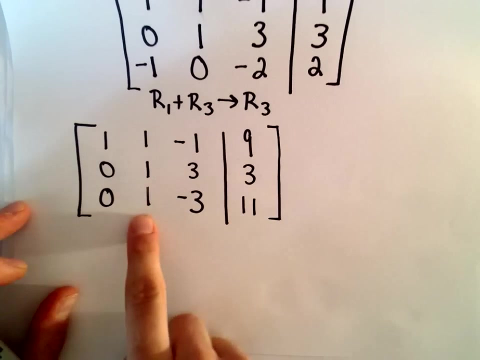 one plus zero will be one negative one plus negative two will be negative three, and then nine plus two will be positive eleven. okay, so again we want ones along the diagonal, again forgetting about the, the column with the constants. well, we do have a one in our second row, second column, so that's. 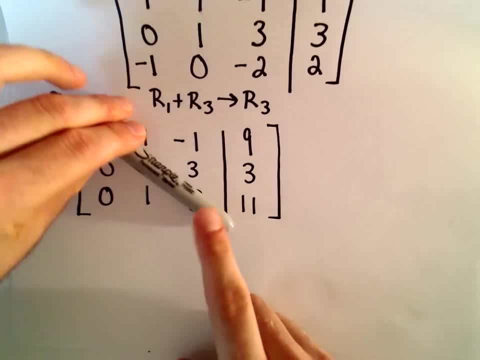 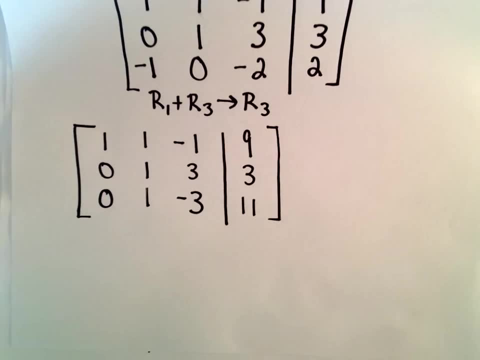 good, we said we wanted to get zeros everywhere below that diagonal. okay, everywhere below that diagonal. so I need to change the entry in the third row, second column. I want to make that into a zero as well. well, if we just add row two in row three, that's not going to do the trick. but if 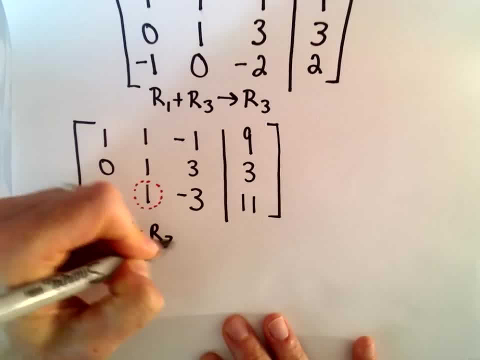 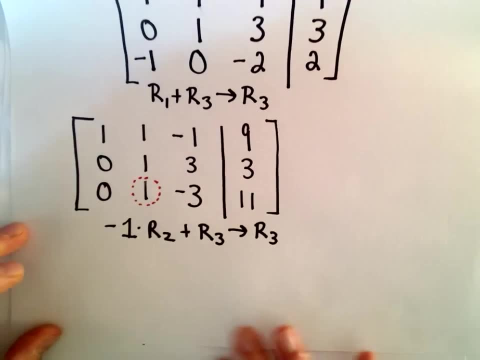 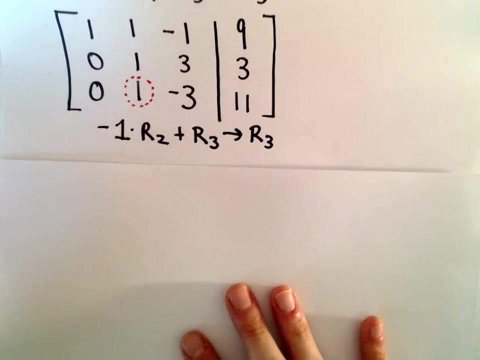 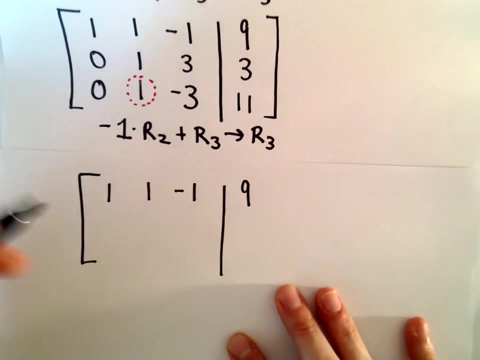 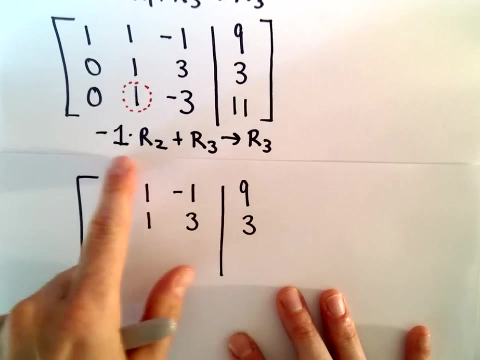 we multiply the second row by negative one and then add that to our third row row. I think that'll do it for us. So let's see here. So again, I'm not changing the first row at all, I'm not changing the second row either. Now I'm going to change the third row again by: 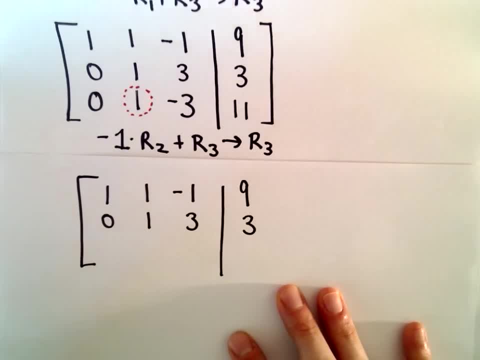 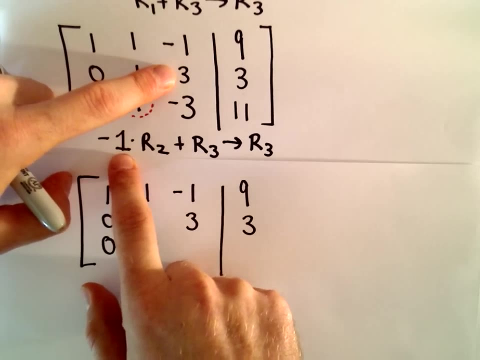 doing the arithmetic. So negative one times zero plus zero, that's just zero. Negative one times one will be negative one. If we add negative one to positive one, we'll get zero, which is exactly what we wanted. Negative one times three is negative three. Negative three plus negative three will give: 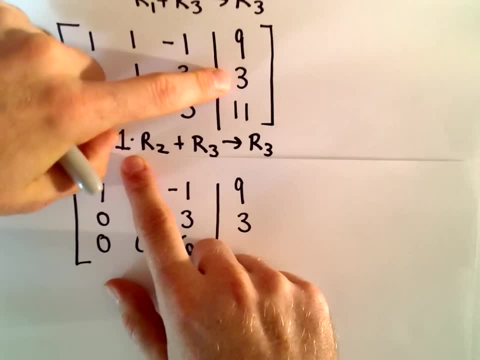 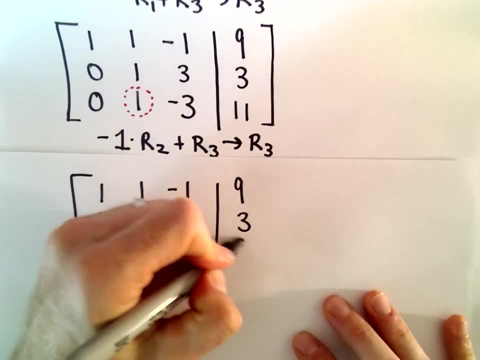 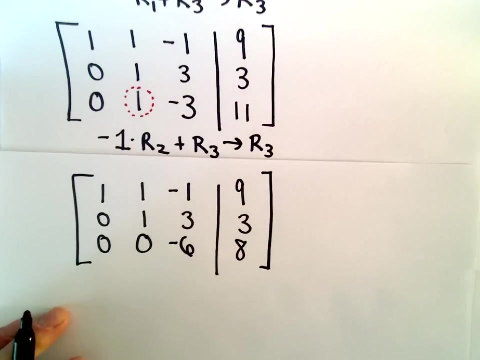 us negative six. Negative one times three again will be well negative. three. Negative three plus 11 will be positive eight, And now we've got our third row All right here getting close. The last thing again we want: 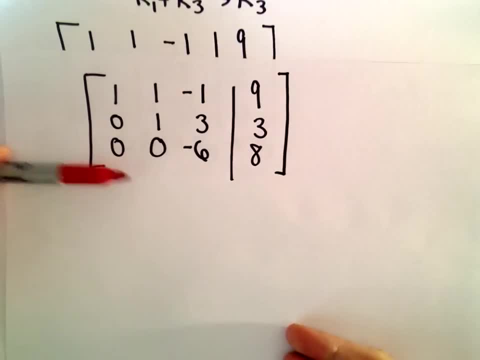 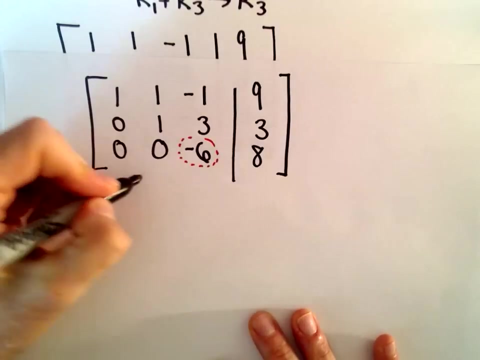 to do is we want to make our first non-zero entry in the third row, which is our negative six. We want to make that into a positive one. Well, what I'm going to do to the third row is simply: you can think, you know I would divide by negative six. 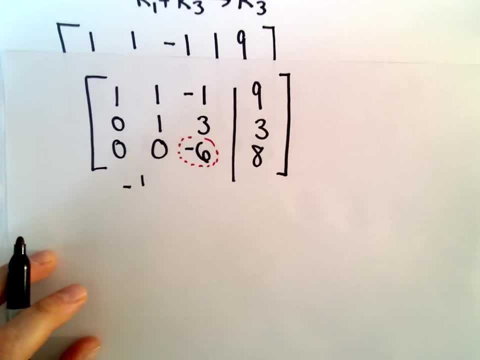 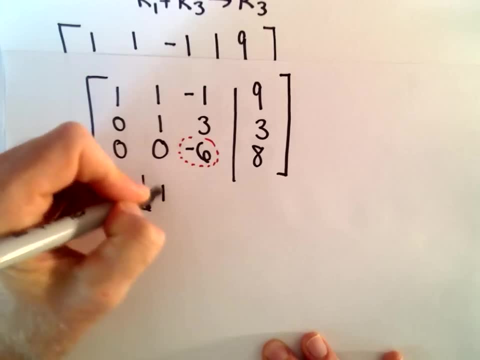 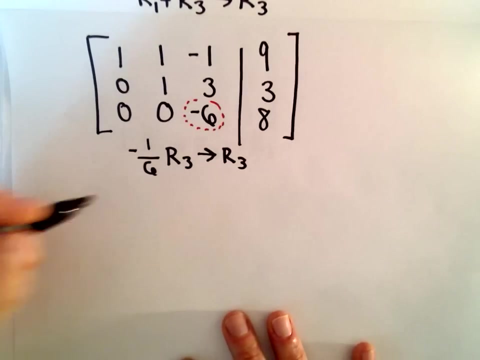 We don't really think about division so much. We always talk about multiplying by non-zero constants. So I'm going to multiply the third row by negative one sixth, And that's going to give me my new third row. So in essence, you're just dividing the third row by negative six Again. 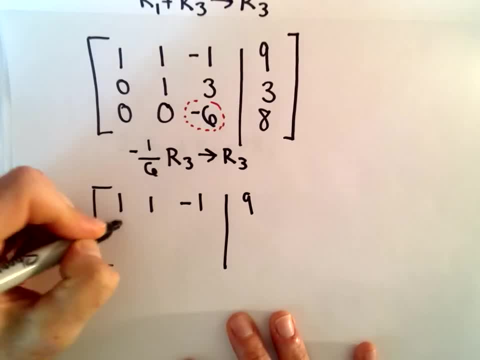 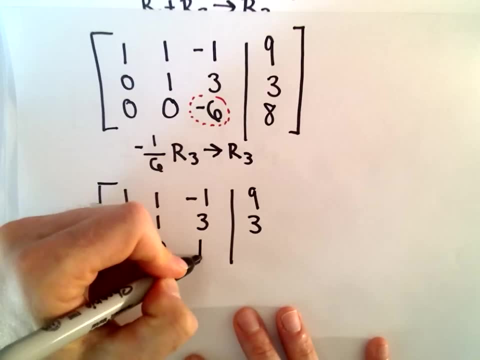 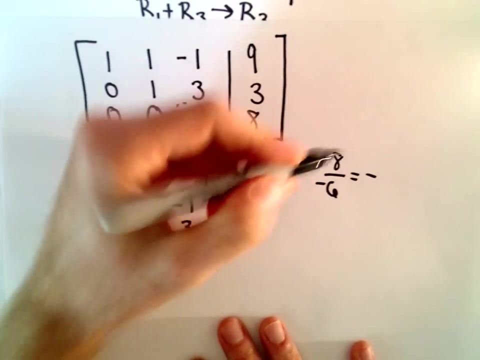 not doing anything to the first row, Not doing anything to the second row. Negative six divided by negative six would be positive one. Eight divided by negative six. well, that would be eight over negative six, And we can reduce eight over six into four-thirds, Again not forgetting the negative. 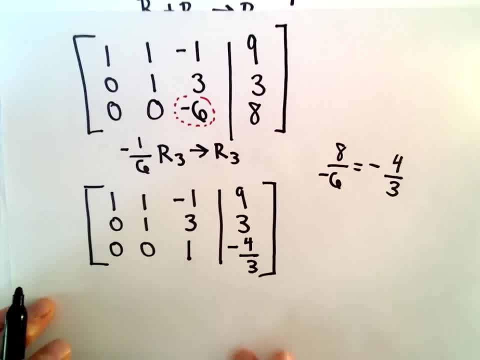 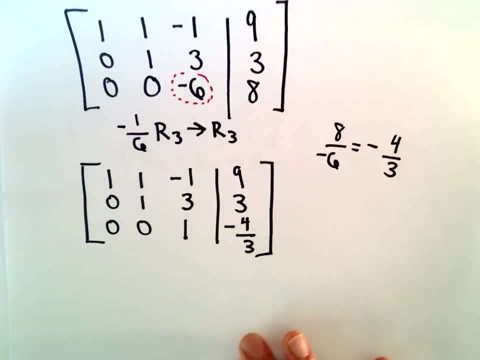 Okay, so now we've got our matrix in the form that we want, And what we do now is we go back and write the corresponding set of linear equations And then we start using substitution- back substitution- to solve, And then we start using substitution- back substitution to solve. 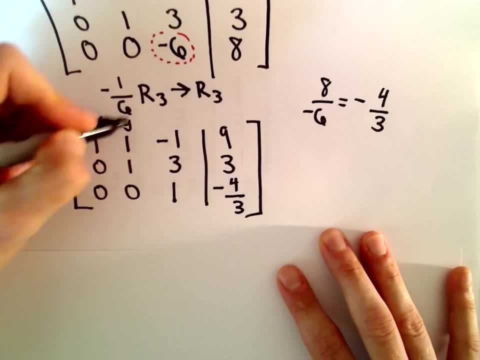 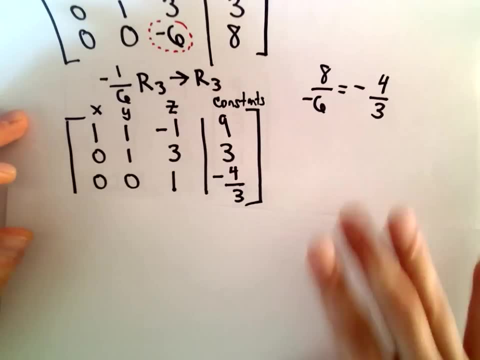 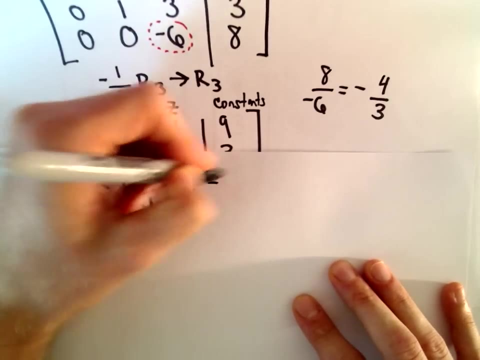 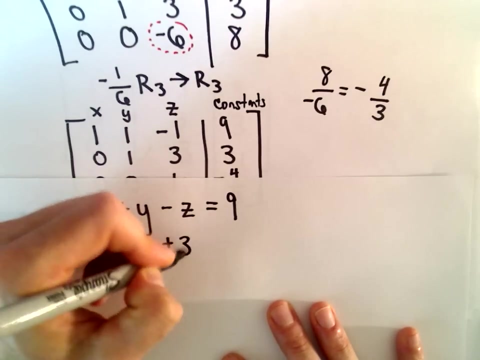 So recall, this is the column corresponding to x, the column corresponding to y, the column corresponding to z, and then our constants. So we've really got the system of equations: one x plus one y minus one, z equals nine. From our second row we've got zero x plus one y plus three, z equals three. 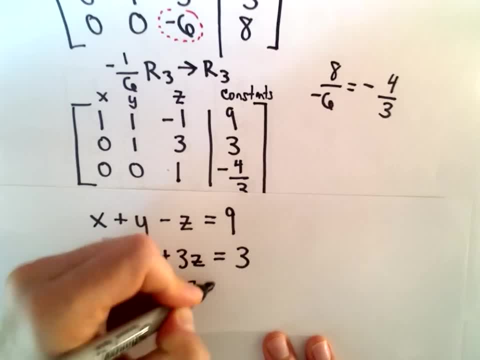 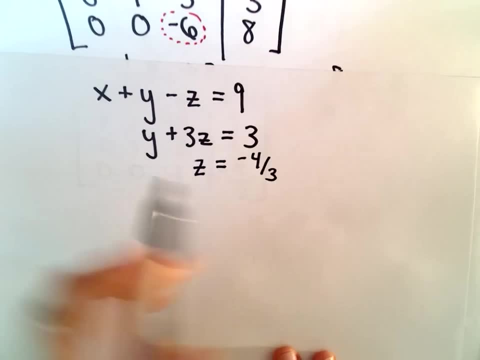 And from our, our last row, we simply have that positive one. z equals negative four-thirds. Okay, so now we know what z equals. The idea is we can take that and substitute that into the second equation, solve for y. Then we'll have both y and z. Then we can substitute that into the first equation and solve for x. 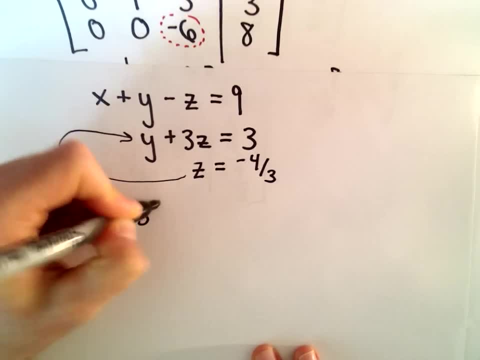 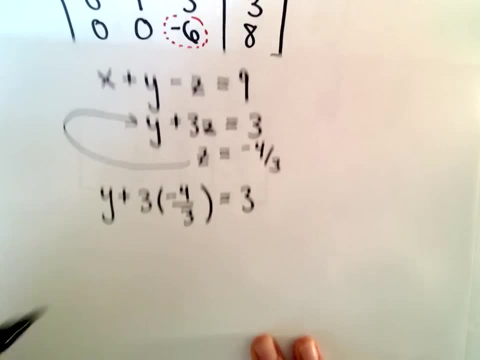 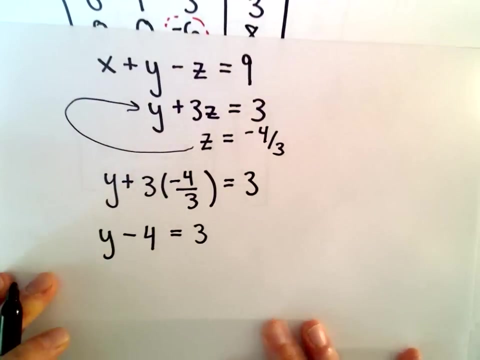 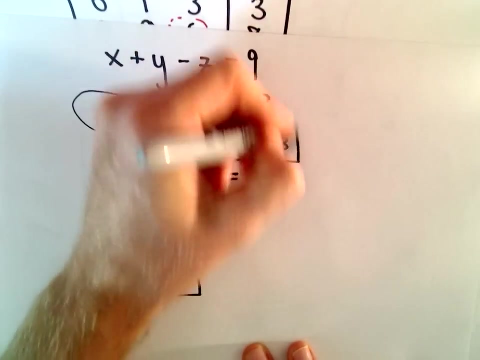 Okay, so using our second equation, we have y plus three times z, That's negative four-thirds. That equals positive three. Well, the three's would simply cancel out, so we would have: y minus four equals three, And if we add four to both sides, we'll get that y equals positive seven. 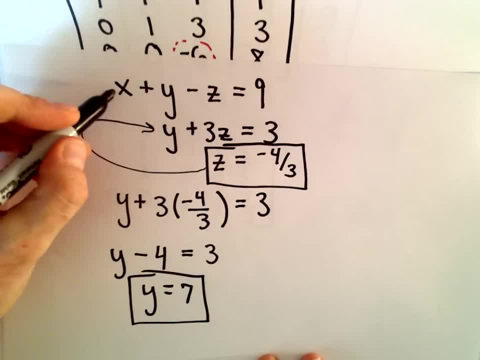 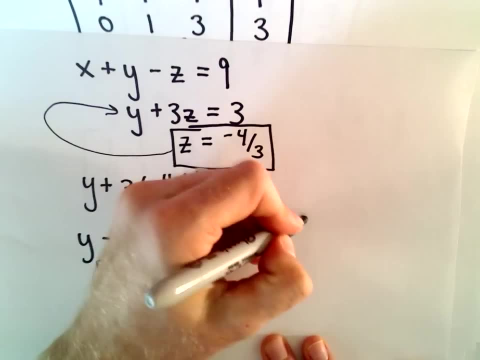 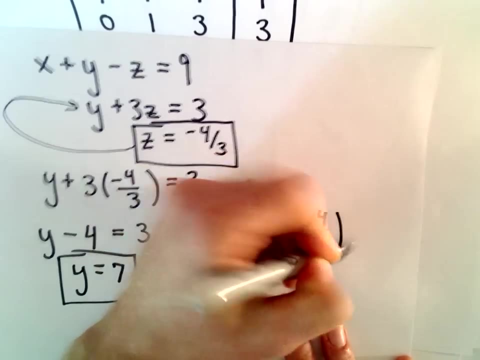 Okay, so now I'm going to take these two values and simply put those back into our first equation. So again we had x plus y, which is 7,, minus the value of z, which is negative 4 thirds, And that's going to equal positive 9.. 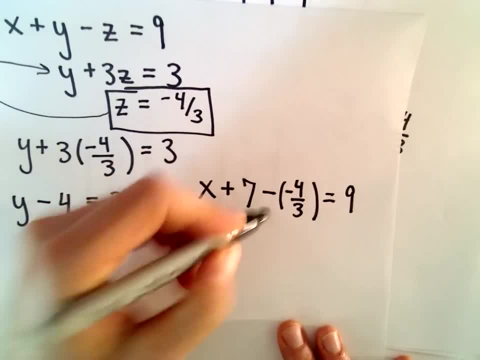 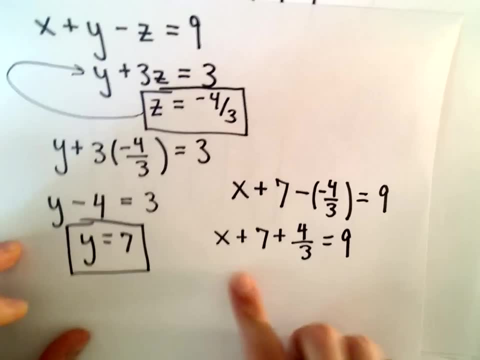 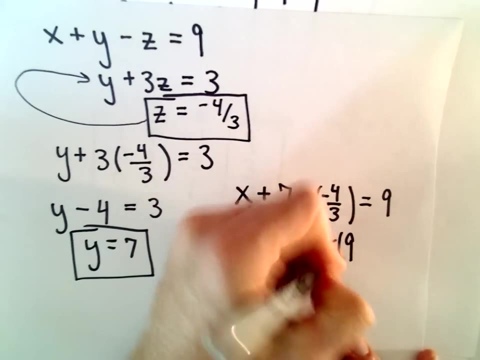 All right, so very close. here We've got x plus 7. We would have plus 4, thirds equals 9.. And you could always get common denominators and add and subtract fractions. I'm going to get rid of the fractions, or I should say fraction, by multiplying both sides by positive 3.. 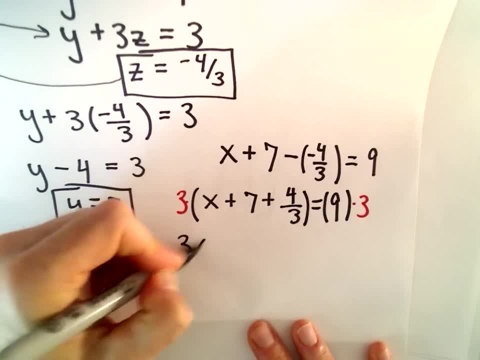 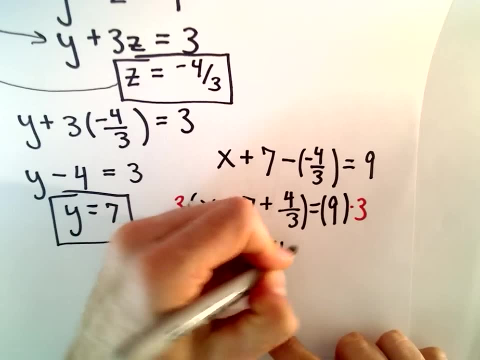 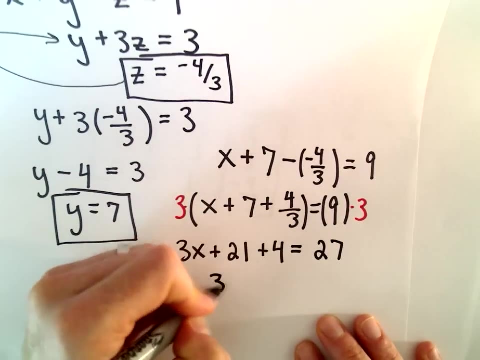 So we'll have to distribute that. We'll get 3x. 3 multiplied by 7 is positive 21.. 3 multiplied by 4 thirds would just be positive 4.. 9 times 3 will be 27.. Let's see: 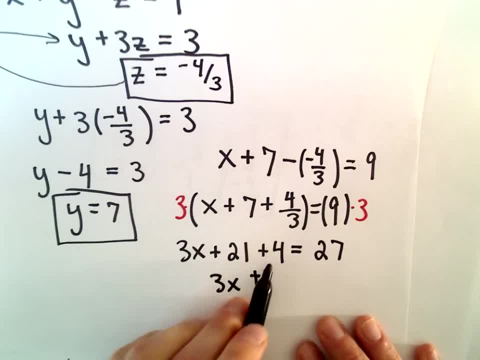 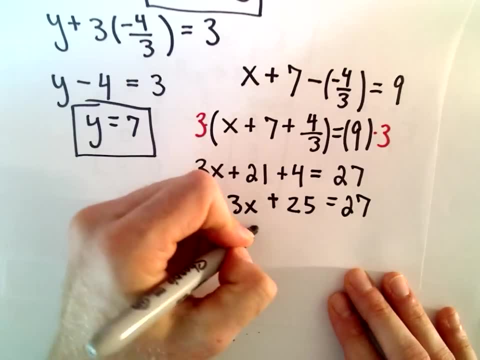 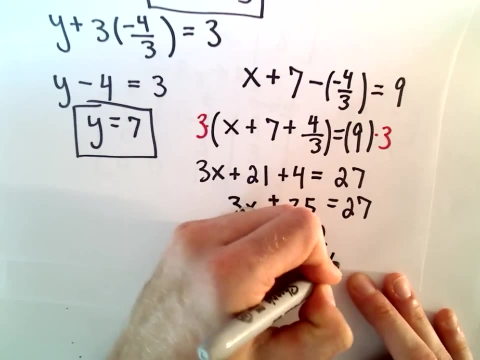 We would have 3x. 3x plus 21 plus 4 will be 25.. And if we subtract 25 from both sides, we'll get that 3x equals 2. And if we divide both sides by 3, we'll get that x equals 2 thirds. 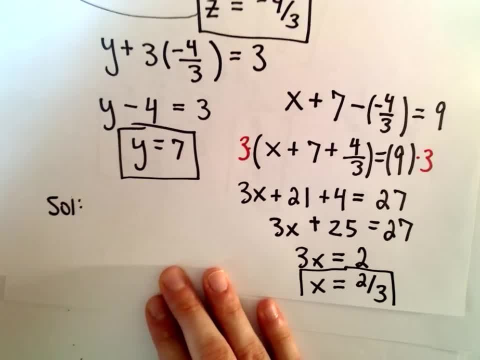 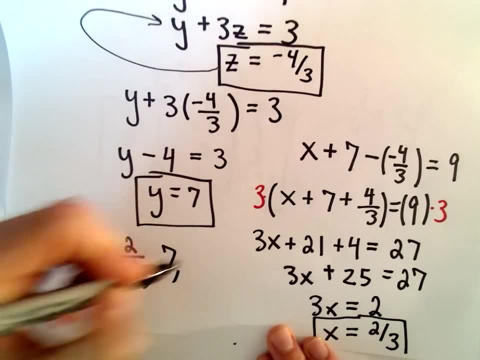 So now we've got our solution. It says the solution to this system of equations would be: when x equals 2 thirds, we said that y equals 7, and z equals negative 4 thirds.